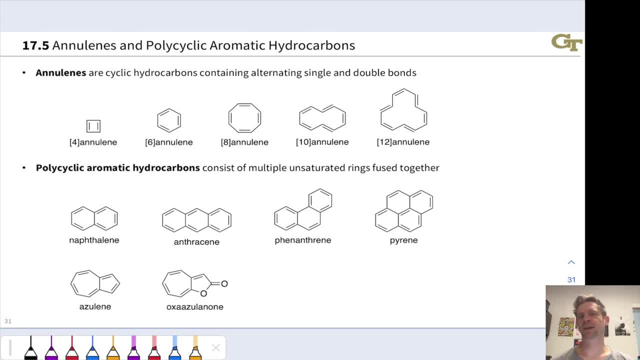 So far, we focused mostly on monocyclic hydrocarbons with one ring that are fully conjugated in the discussion of aromaticity and anti-aromaticity. In this video we're going to look at other types of aromatic compounds: anulenes- polycyclic aromatic hydrocarbons. 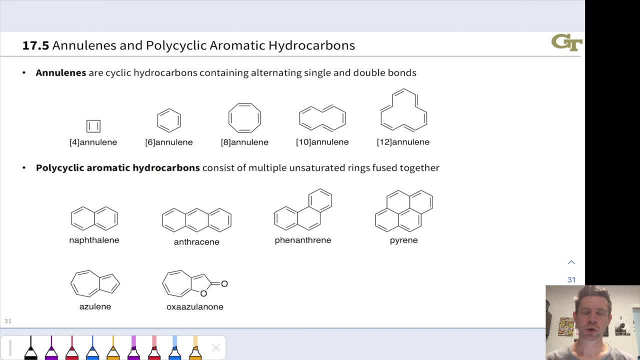 and aromatic heterocycles containing a heteroatom within the ring. Let's start with anulenes. And anulenes may be aromatic, anti-aromatic or non-aromatic if they're in the non-planar conformation. Anulene is just a generic term for a cyclic fully conjugated hydrocarbon consisting 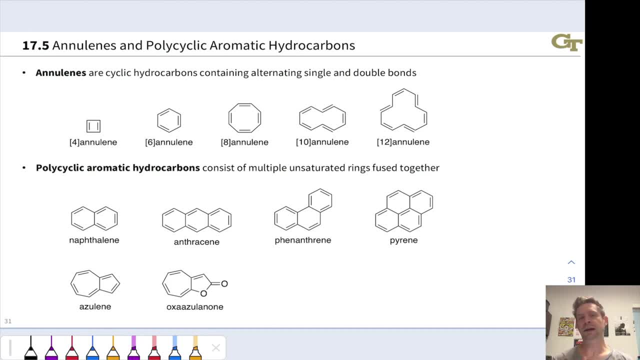 of alternating single and double bonds And we put a number out in front in brackets, in square brackets, indicating the size of the ring of the anulene. So, for example, cyclobutadiene is equivalent to four anulene with four atoms in the ring. Benzene is equivalent to six anulene and 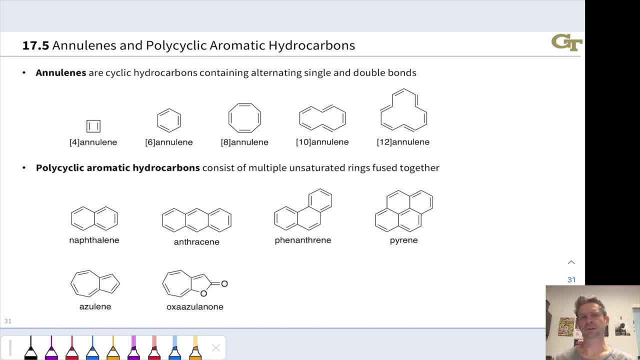 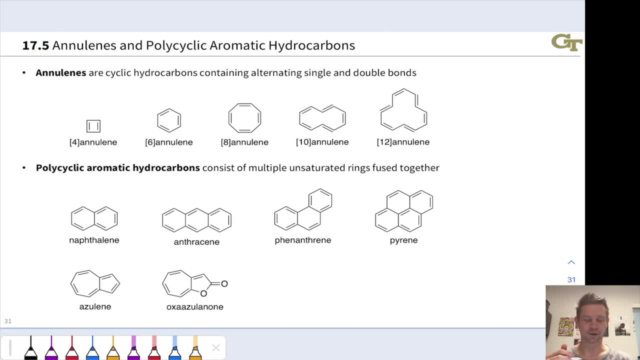 get to ring sizes of six. And when you get to ring sizes of six you get to ring sizes of six, So let's say nine or higher. where the names get awkward, right Naming gets awkward. So, for example, 10-anulene is just a fully cyclic conjugated hydrocarbon. fully conjugated. 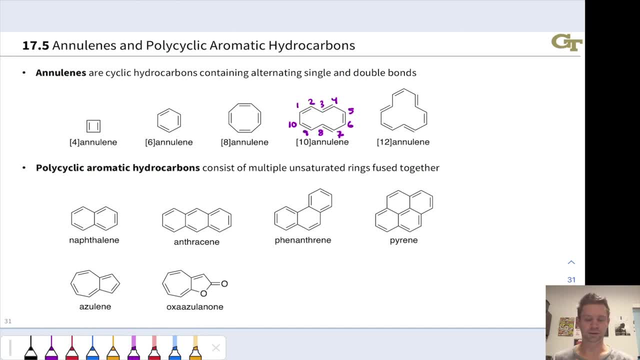 cyclic hydrocarbon with 10 carbons in it, with alternating single and double bonds, And if we count the carbons around the ring here, we see that there are indeed 10 carbons, And these can have cis-trans or EZ issues as well. Generally, we're not going to worry about those, but that's. 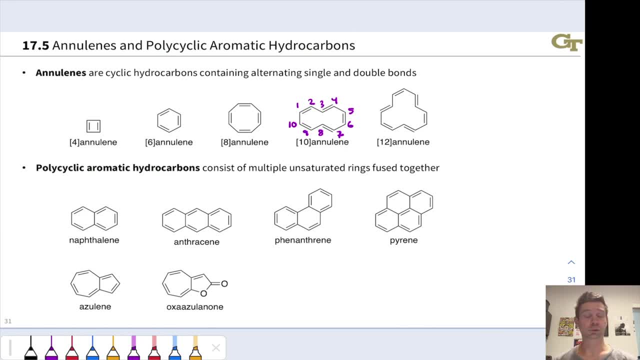 worth thinking about in these larger ring sizes in particular, that double bonds can be either cis or trans Polycyclic aromatic hydrocarbons contain more than one aromatic ring fused together, And by fused here we mean that two rings are sharing a bond. So, for example, 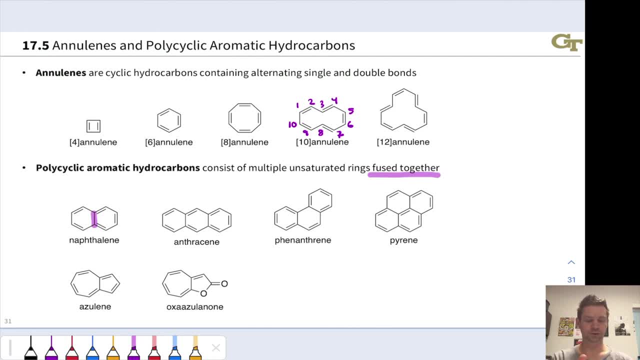 in naphthalene. naphthalene looks like two benzene rings fused together, with this bond highlighted in purple shared between the two benzene rings, And naphthalene is aromatic, and that's actually worth verifying on your own. Pause the video and verify that this. 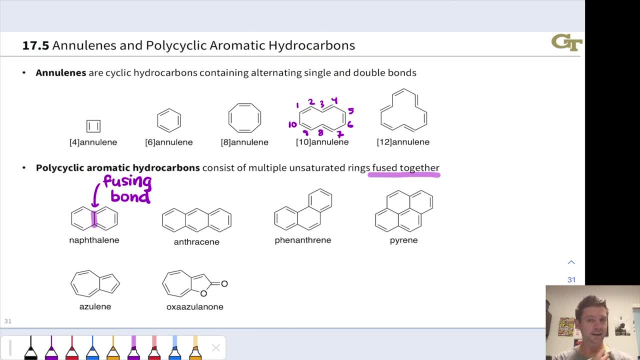 molecule is aromatic, It is cyclic, it's fully conjugated, it's planar and it does contain a Huckel number of 4n plus 2 pi electrons. The other examples: we can have more than two rings fused together, For example in anthracene. those three rings can be fused together in a linear way. 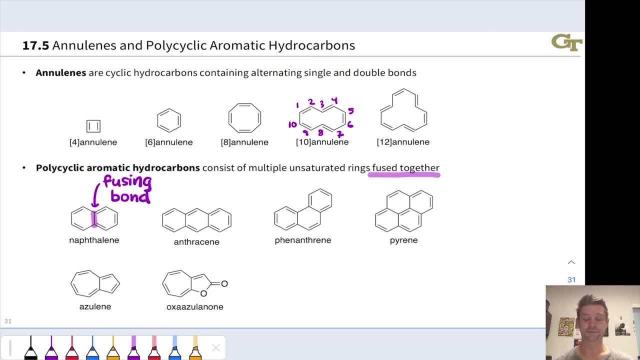 in anthracene or in kind of an angular way. That's what's going on in phenanthrene. We can have rings fused along multiple bonds. So for example, in pyrene, this ring here has a fusing bond. here, here and here Get this kind of honeycomb shape. Azulene and oxazulonone- here are what are. 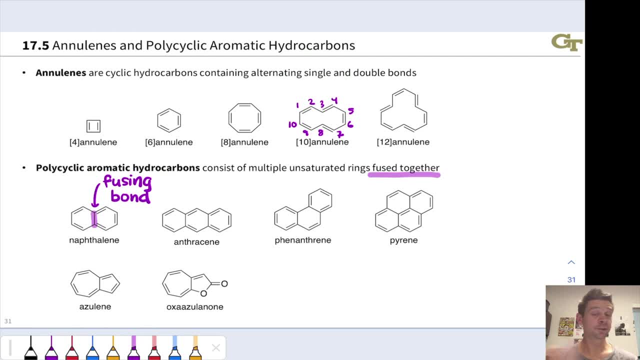 known as non-benzene-moid aromatic compounds because they don't contain benzene rings. All of these top four structures. we can find benzene rings within the structures, right, If we look individually at the rings, they're six-membered. they look like benzene rings. Azulene has a 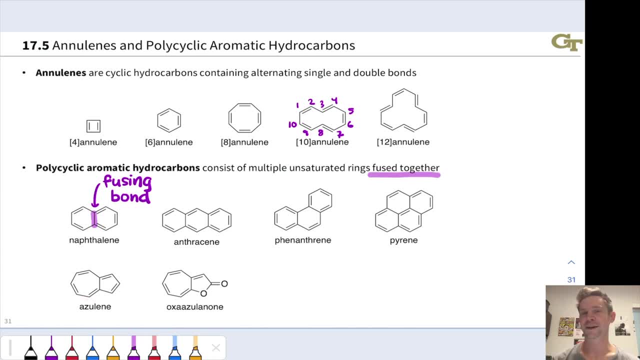 seven-membered and a five-membered ring and is a really interesting compound that actually exhibits polarization. I won't get into that in any more detail And oxazulonone is technically a heterocycle, but I wanted to highlight it because it may not appear. 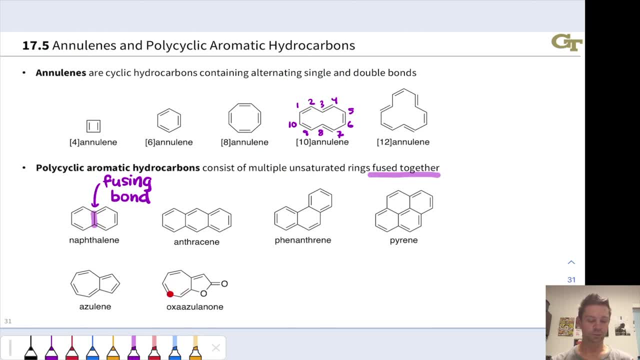 aromatic. After all, if we just count the pi bonds, I've got two, four, six, eight electrons. This kind of looks anti-aromatic, but don't forget that heteroatoms can participate in pi systems as well And an alternative resonance form of this molecule involving pushing these this lone. 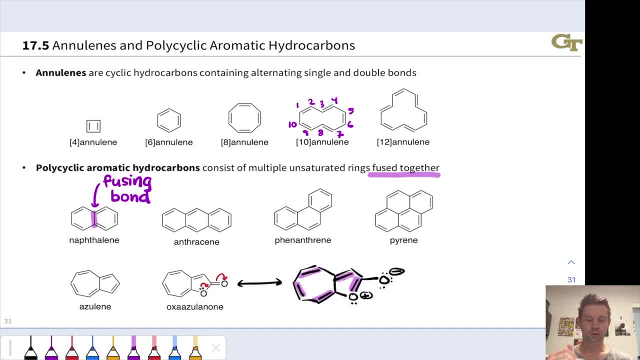 pair on oxygen into a pi bond with the carbon next door shows that in fact there are two, four, six, eight, ten pi electrons in this resonance form, showing us that this molecule is in fact aromatic as a result of the ten pi electrons. 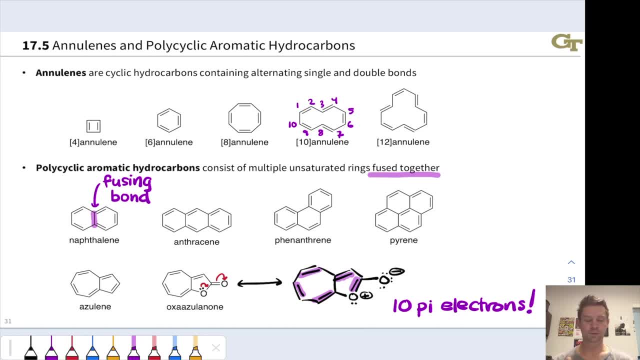 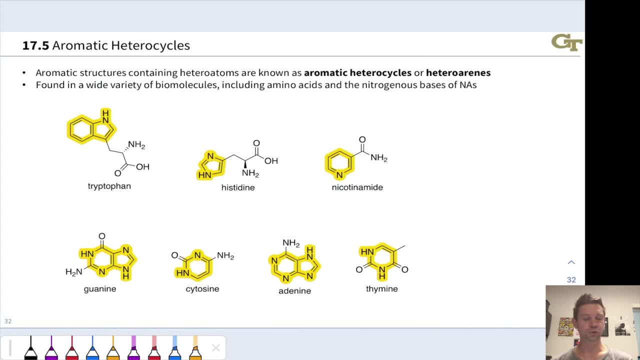 So on this slide we looked at anulenes and polycyclic aromatic hydrocarbons. Recognition that this oxygen is participating in the aromaticity of this molecule is a nice segue into aromatic heterocycles, Hugely, hugely important, Found in a wide variety of compounds, For example: 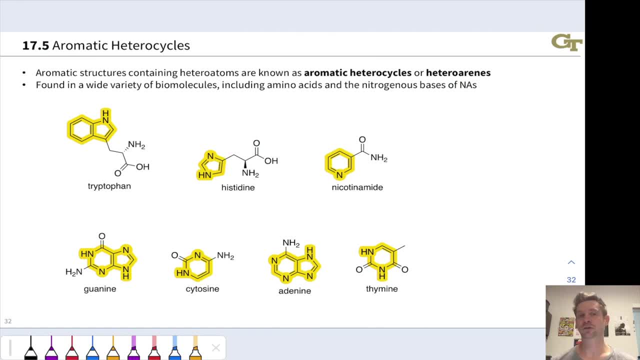 in biochemistry, and this slide features compounds that are biochemical, containing aromatic heterocycles. So, for example, in the top left here we see a five-membered ring containing nitrogen fused to a benzene ring. This whole system, highlighted in yellow, is known as the. 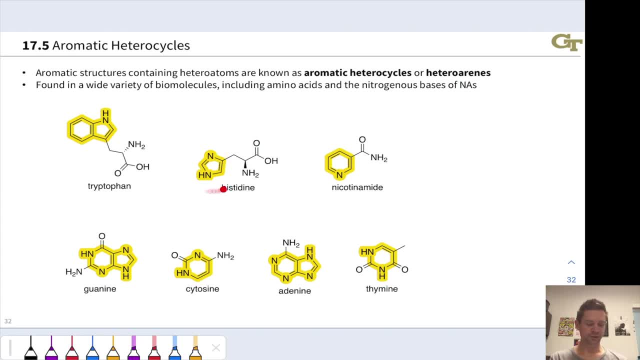 indole system. We have two nitrogens in this five-membered imidazole ring and histidine, and these two compounds, tryptophan and histidine, are natural amino acids. The nicotinoids, or nicotinamide group, or nicotinamide molecule, contains what's called a pyridine ring, six-membered. 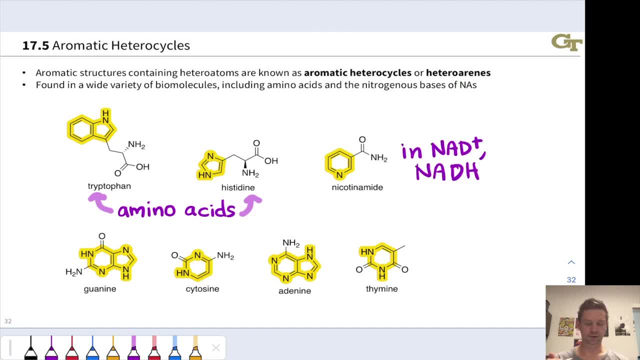 ring with nitrogen, and this is very important because it's found in NAD plus and NADH. These are biochemical cofactors used for oxidation and reduction respectively, and we'll see them when we discuss those topics later in the course. in 2312 LS, The four molecules 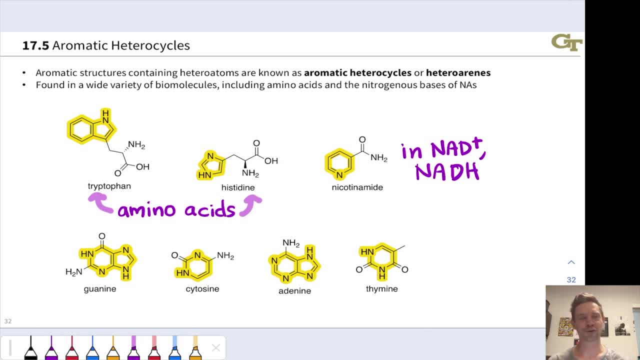 along the bottom are probably the most important and well-known nitrogen-containing heterocycles in biochemistry. These are the nitrogenous bases. We see a large number of nitrogen atoms in the rings of these structures, all of which are aromatic. All of these highlighted ring systems are aromatic, so aromatic rings are. 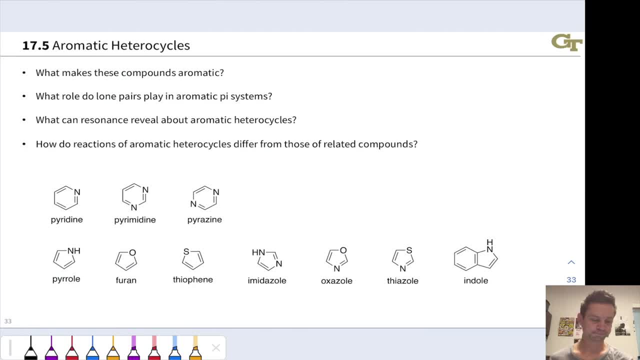 hugely important in biochemistry and well beyond, of course. With aromatic heterocycles, some interesting questions arise. The basic question of what makes these compounds aromatic. Actually, Huckel's rule and all of those criteria that we've seen previously still apply. 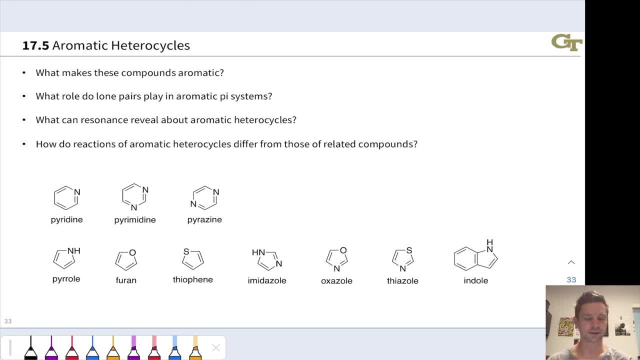 But there are some interesting questions about how these compounds are aromatic. There's some wrinkles with the lone pairs brought in by heteroatoms. We want to know what role do those lone pairs play? Are they part of the aromatic pi system or not? Are they basic? 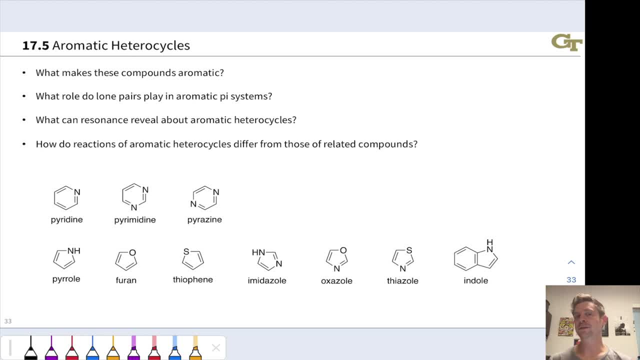 or Bronsted or Lewis, basic or not? What can resonance reveal about aromatic heterocycles? Those heteroatoms exert interesting effects by pushing or pulling electrons and we can pick that and understand that using resonance. And then finally we'll think about aromatic heterocycles and reactions. How are they similar? 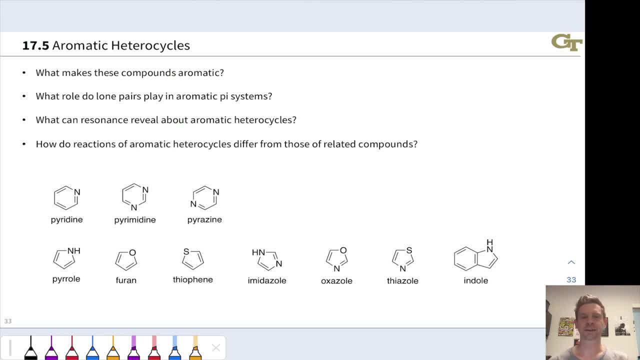 to aromatic hydrocarbons and how are they different? We're going to keep that question at the top of our minds moving forward as we move into aromatic reactivity. The bottom of this slide highlights some examples of common heterocycles. I won't go through. 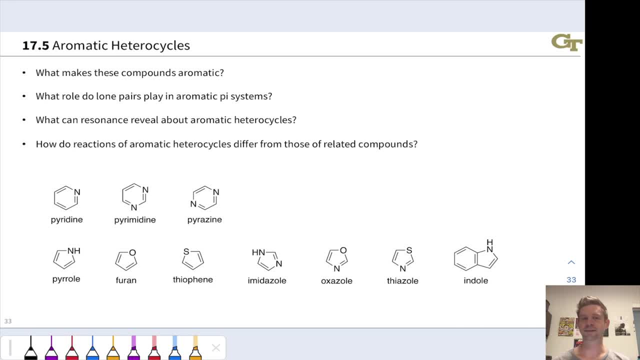 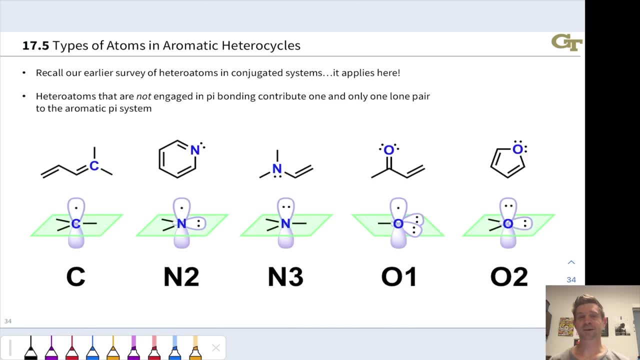 all the names, but it's a good idea to familiarize yourselves with these names again, just to make reading and studying organic chemistry easier as you move forward. Aromatic heterocycles are conjugated systems, so now is a good point to recall our coverage. 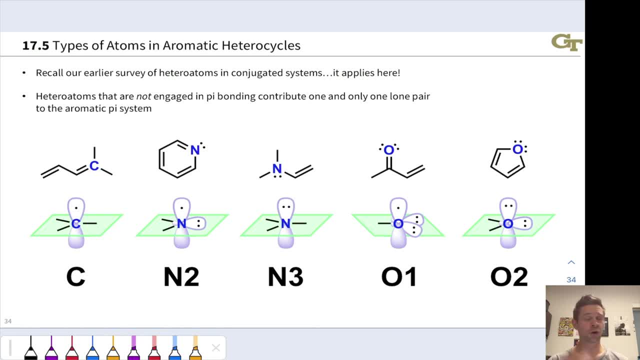 the structures of heteroatoms within conjugated systems. All of those ideas apply here in the context of aromatic heterocycles. We want to keep in mind, for example, that heteroatoms that are not engaged in pi bonding can contribute one and only one lone pair to the aromatic. 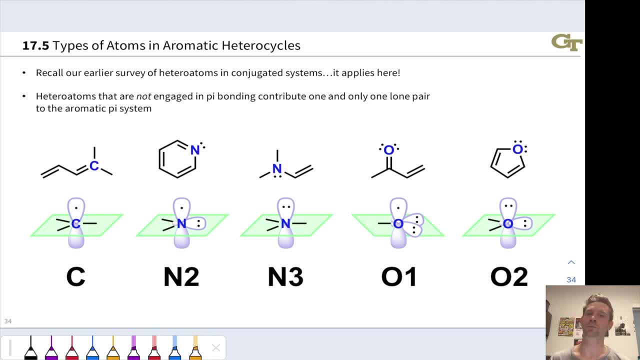 pi system and a given heteroatom can never contribute more than two electrons to a pi system. It's still true in a heteroaromatic context and in fact this ring right here. pyridine is an aromatic heterocycle. Let's walk through this listing of atom types in. 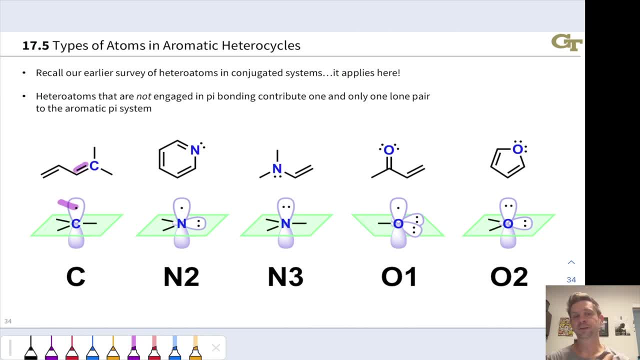 conjugated systems one more time. First, we've got the carbon, and carbon is typically involved in pi bonds in conjugated systems and heterocycles, aromatic heterocycles and aromatic hydrocarbons. Carbon typically contributes one pi electron via its pi bonding with an atom next door. 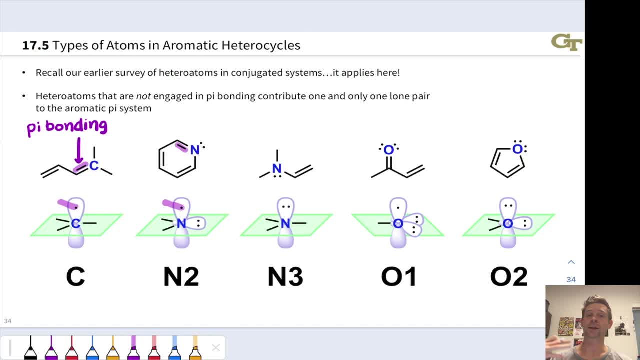 The N2 nitrogen, remember, is involved in pi bonds. It contributes one pi electron via that pi bond and the lone pair is not involved in the aromatic pi system. This is not pi electrons and it's free to be donated as a Lewis or. 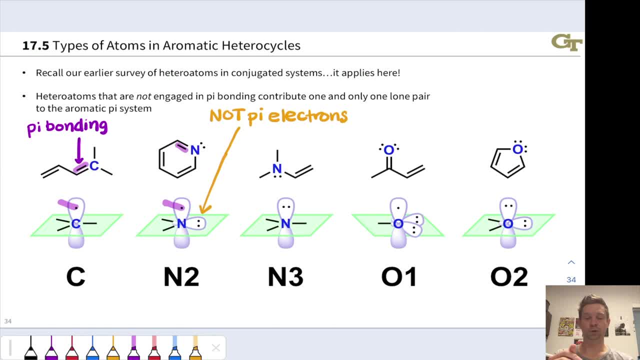 Bronsted base. as a result, The N3 nitrogen has a lone pair that is part of the pi system. however, We know this because that nitrogen is not involved in pi bonding- three single bonds- and so this lone pair can occupy a p orbital, and it will do so when there is 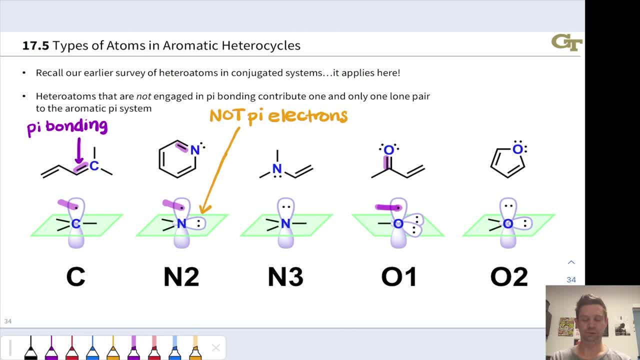 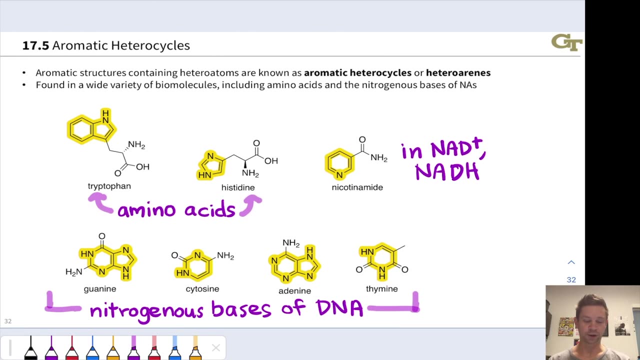 a double bond next door, or a p orbital next door more generally, such that it can delocalize itself. like so, The O1 oxygen has a pi bond, that's a carbonyl oxygen, and this you won't find inside a heterocycle but it may be attached to an aromatic heterocycle, For example if 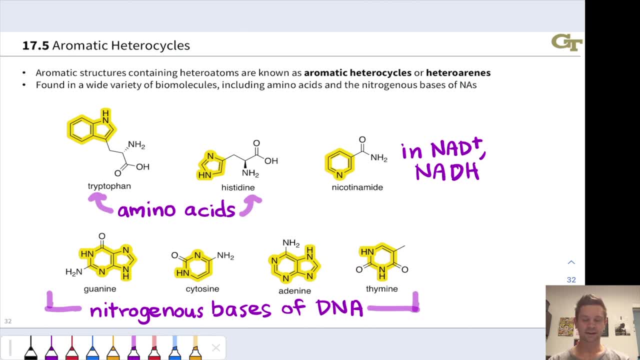 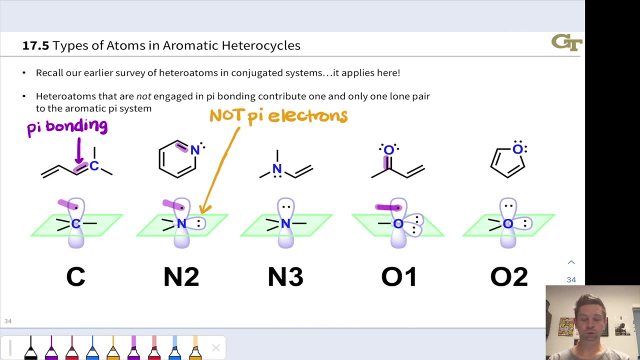 we look at thymine, this O1 oxygen is in conjugation, we would say with the ring highlighted in yellow. It's got a p orbital, that oxygen that is overlapping with the p orbital cell on this carbon. here The O1 oxygen contributes one pi electron and its two lone pairs are: 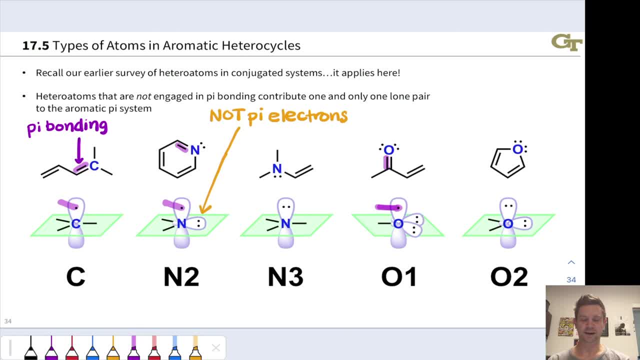 part of the sigma system, not the pi system. Those are not pi electrons. Similarly, with the O2 oxygen, it has one lone pair. now that is not part of the pi system, but because it has only single bonds, no pi bonding, this lone pair is capable of occupying a p orbital.